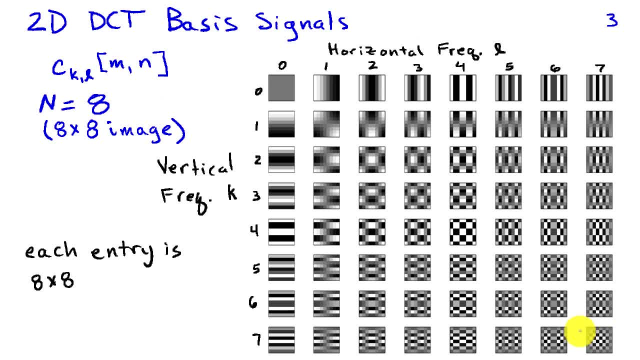 that represent the 64 pixels in an 8 by 8 image. So in this first column we're seeing the vertical cosine And in the first row we're seeing the horizontal frequency cosines, and then in the other entries we're seeing products of these different horizontal and vertical frequency cosines. 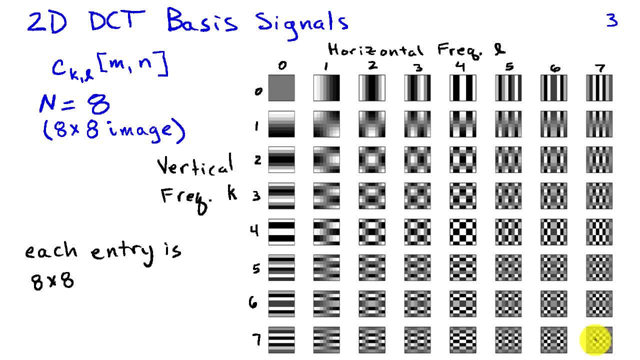 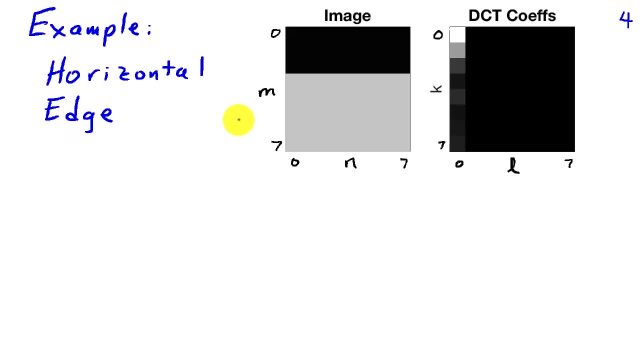 with the lower right corner being the product of the highest frequency horizontal and vertical cosine. So, for example, the basis image associated with k equals 5 and l equals 2 is circled and green. In this example, we're showing an 8x8 image which consists of a horizontal edge. 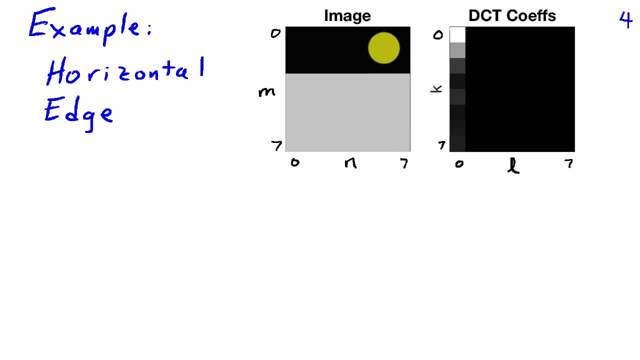 So we're going from light gray to nearly black and if we take the DCT coefficients of this image, we find that they're all concentrated in the L equals zero or along the vertical frequency direction. So they have zero horizontal frequency, which is consistent with the fact there's no 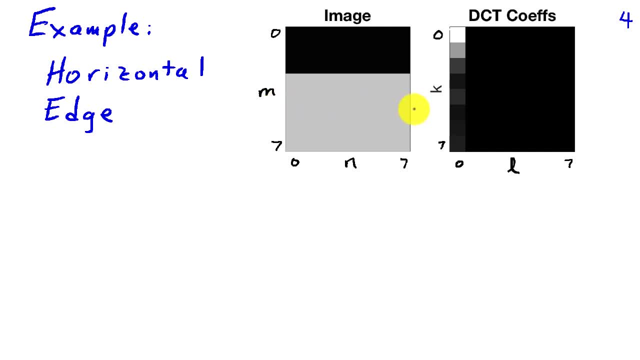 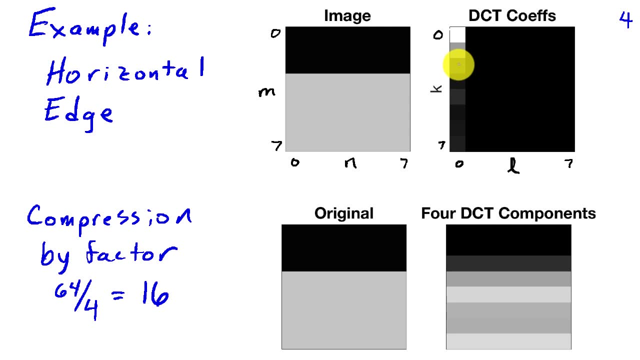 variation in this image in the horizontal direction. Now, the idea of image compression is to use only a portion of the coefficients. So, for example, all of these coefficients on the right-hand side, they're all zero And in the example I'm showing below, we used only four of. 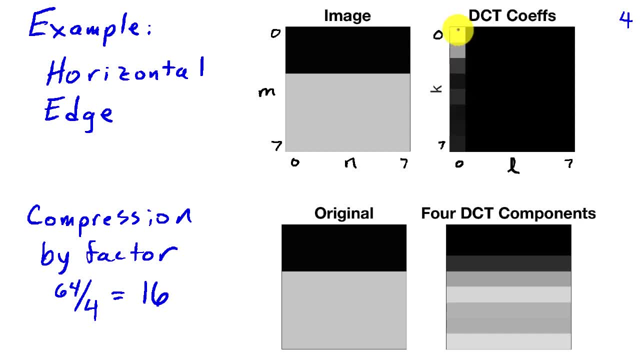 the DCT coefficients- this one and these three, which were the four largest- And if we approximate the image using only the DCT coefficients, we're going to have zero. So we're going to have zero and we're going to have only four DCT coefficients. We see that we do a pretty good job of. 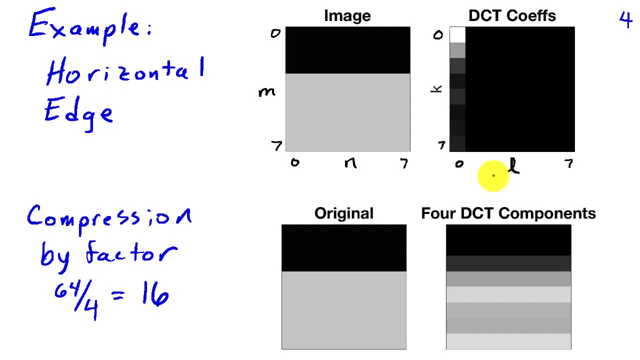 reconstructing the edge and since we're using four DCT coefficients as opposed to the 64 that were originally present, we've achieved compression by a factor of 16, or 64 over 4.. In this particular image, since it has this horizontal edge and therefore all of the horizontal DCT coefficients, 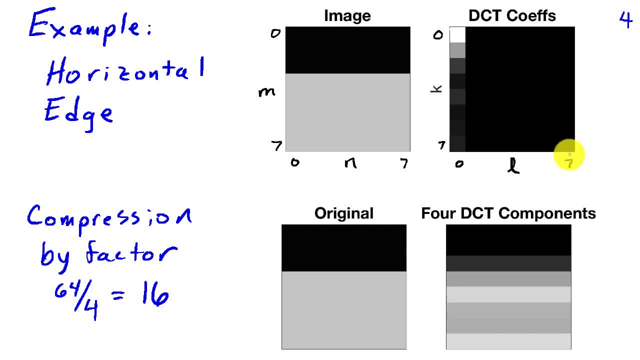 with L equal 1 through 7, we're going to have zero. So we're going to have zero. And since we're going to use only the L equal 0 terms, we could have perfectly reconstructed the original image using only eight DCT coefficients, So we could have got a compression by a factor of 8 with no. 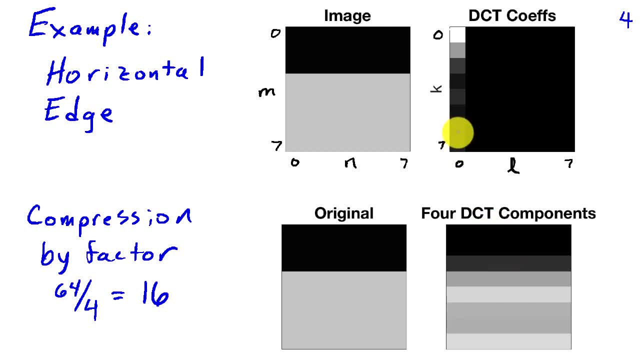 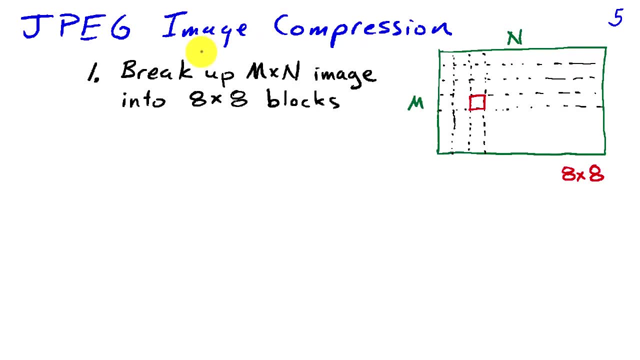 loss or no approximation error by using all of these eight coefficients, And this is the basis behind JPEG. In JPEG, when we compress an image, we're going to break up some arbitrary large m by n integers And we're going to have zero. So we're going to have zero, And since we're 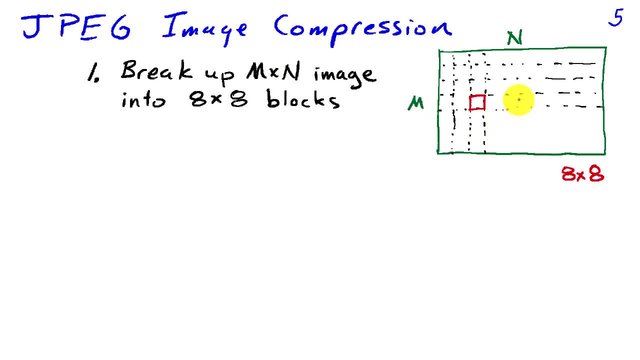 image into 8x8 blocks, as I've illustrated in this graphic. Then for each block we take the two-dimensional discrete cosine transform to find the DCT coefficients corresponding to that block And we save the important and significant DCT coefficients. That's based on the size of the 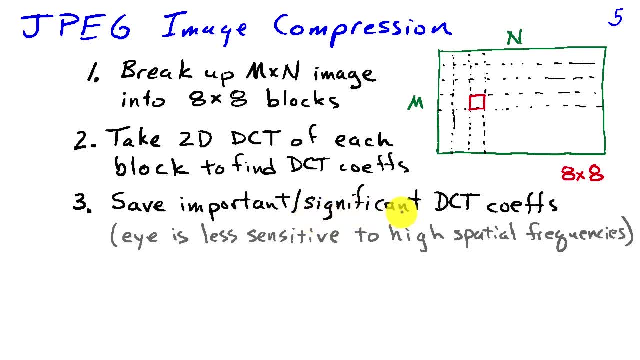 coefficients as well as the importance of them to a human viewer, Because the human eye, it turns out, is less sensitive in general to high spatial frequencies. So a DCT coefficient associated with very high spatial frequencies would need to have a larger amplitude to be as important as one. 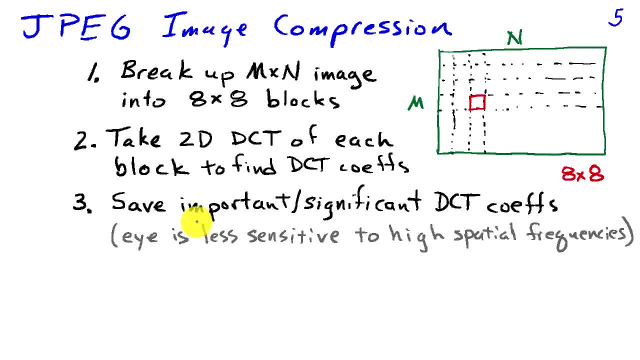 associated with the lower spatial frequencies. Now, in practice, rather than just thinking about saving or discarding DCT coefficients, what happens is that bits are allocated to each DCT coefficient Based on its significance or importance. If a particular coefficient is deemed more significant, 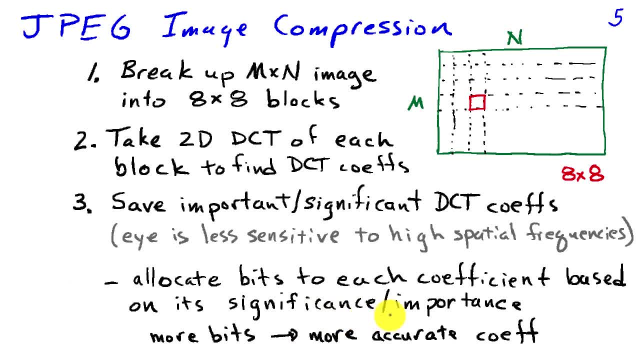 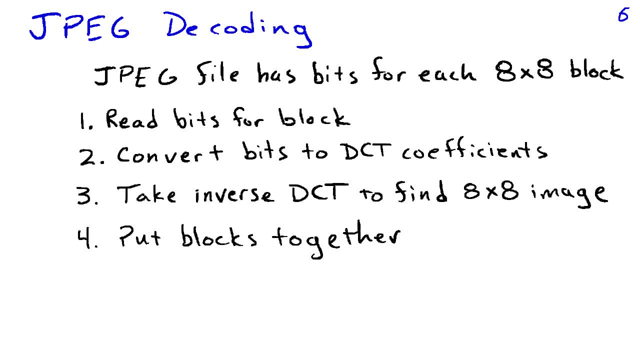 and important, we would allocate more bits to that coefficient. This again is based on the size or amplitude of the coefficient, as well as the corresponding spatial frequencies and how humans perceive those frequencies. So if we've stored our image in the JPEG format, we can decode it for. 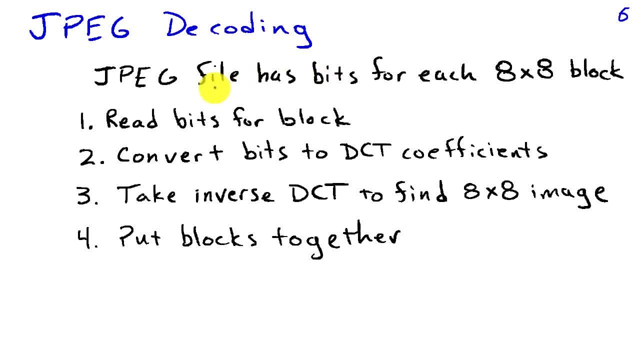 display by reversing the process. So we're going to have the file. there are bits in it for each of the 8x8 blocks. So we're going to read the bits for that block and then convert those bits to the DCT coefficients for that block. 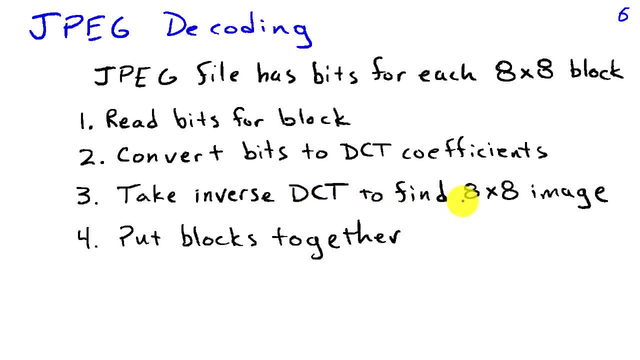 We'll take the inverse discrete cosine transform to find the 8x8 image associated with that block And then, having done that for all the blocks in the image, we simply stitch the individual 8x8 blocks back together to form the complete image.